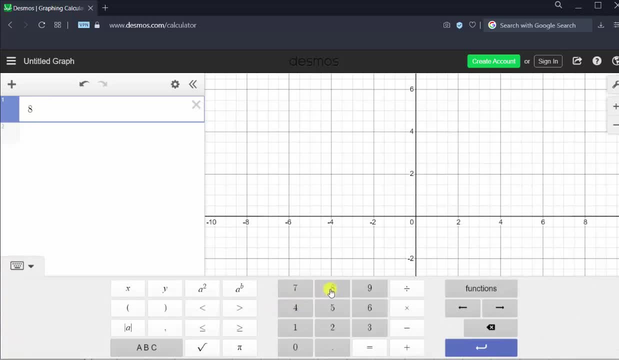 Eight. the exclamation mark is in the letter keyboard. We access the letter keyboard by clicking the large ABC in the lower left-hand corner. The exclamation mark is here in the lower left. Notice how eight factorial is equal to 40,300. 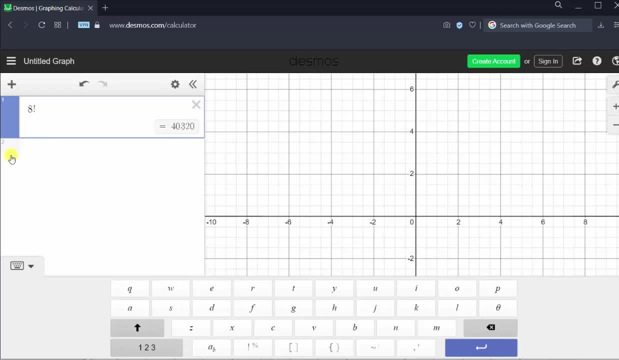 That's 20.. And now to evaluate eight permute five in cell two. We click in cell two and there's two ways to do this. We can enter lowercase n, capital P, lowercase r and then, in parentheses, eight comma five. 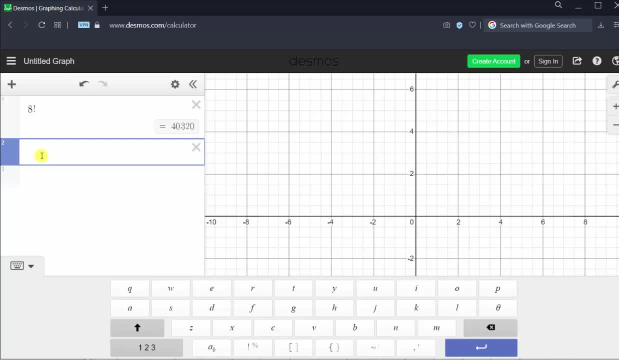 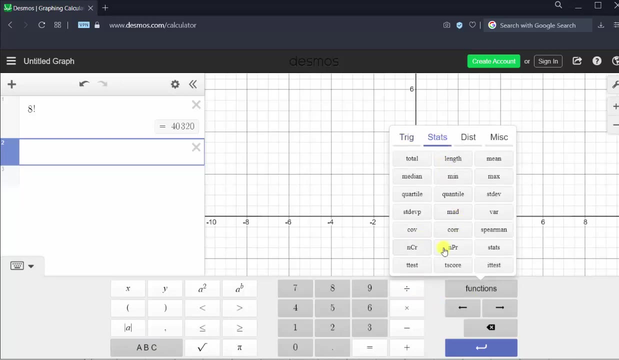 or we can use the functions menu. Let's first use the functions menu by going back to the number keypad, by clicking on the large 123 in the lower left-hand corner, Then click functions, Then click functions, Then click stats Down here toward the bottom. 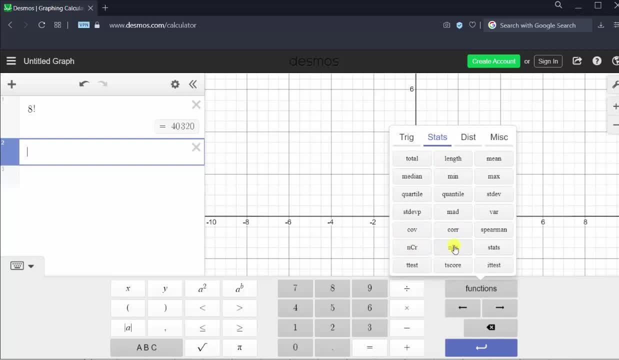 we have the combination function and the permutation function. Let's select the permutation function and then we enter eight comma five in parentheses. So eight comma five, Eight permute five, is equal to 6,720.. Or again, once we know this function, 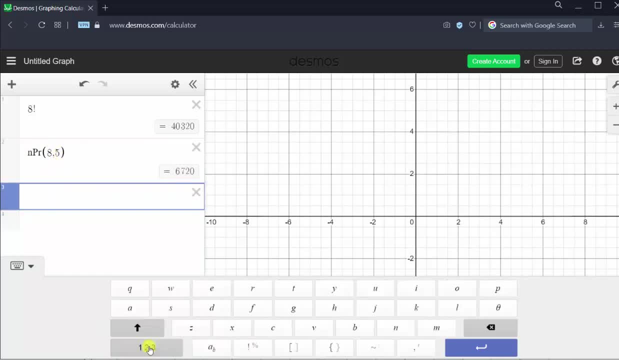 if we go down to cell three, we can, from the letter keyboard, enter lowercase n, capital P, lowercase r, go back to the number keypad and in parentheses enter eight comma five and get the same results. Eight permute five is equal to 6,720. 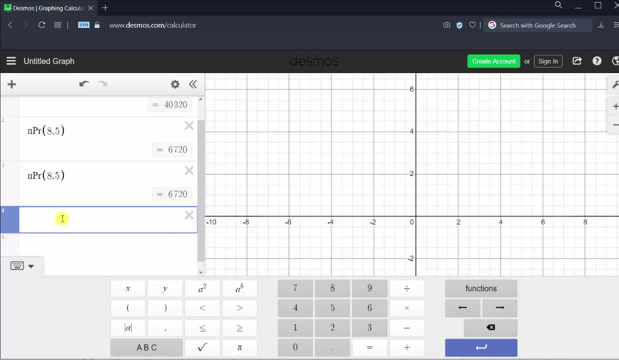 And now let's evaluate: eight choose five. Let's click in cell four. Let's use the functions menu. So we click functions and select the combination function in the lower left-hand corner And then we enter eight comma five. eight choose five. 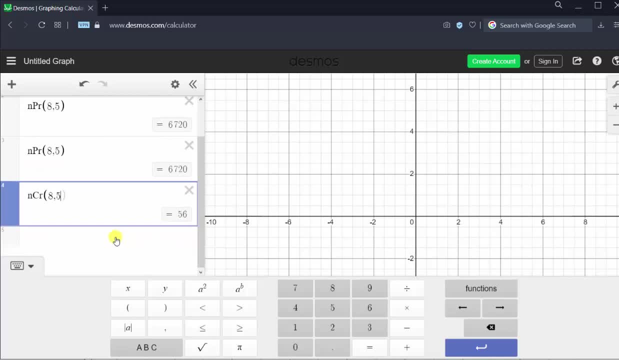 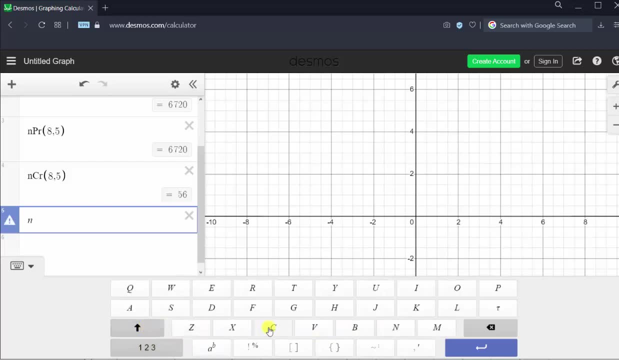 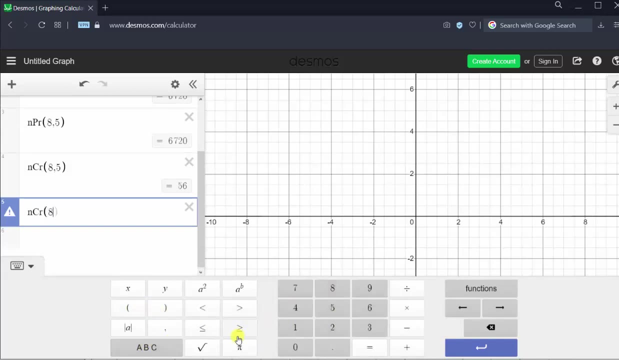 Eight choose five is equal to 56.. Or we can also enter in cell five, go back to the letter keypad, lowercase n, capital C, lowercase r and in parentheses enter eight comma five and get the same results. Eight choose five is equal to 56.. 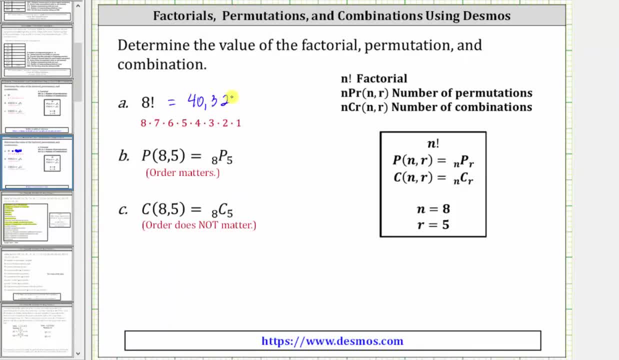 Let's go ahead and record these values. I hope you found this helpful.